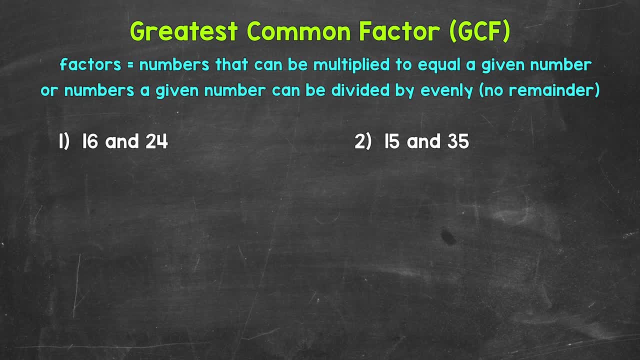 these examples will help you better understand greatest common factor and least common multiple, also known as GCF and LCM. Let's start with greatest common factor. Now, as far as the greatest common factor between numbers, this is going to be the largest factor in value that both 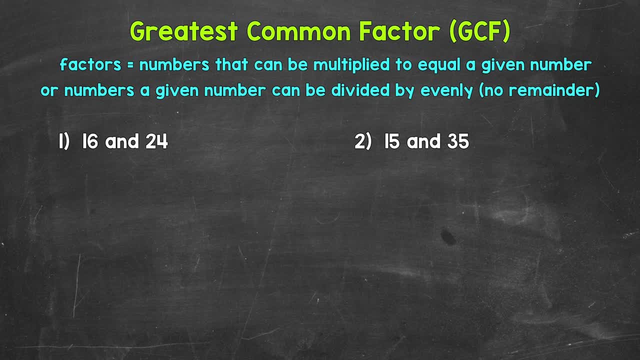 numbers share. Factors are the numbers that can be multiplied to equal a given number. Or you can think of factors as the numbers a given number can be divided by evenly, so divided with no remainder. Now, it's not the most technical or mathematical way to word it, but you can think of factors as the numbers. 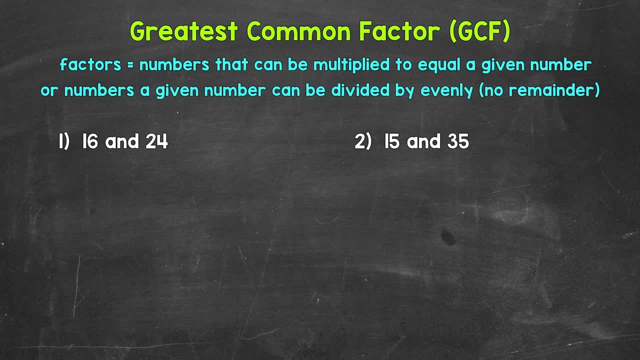 that go into the given number. So again, the greatest common factor is going to be the greatest or largest factor in value that both numbers share, that both numbers have in common. Let's jump into a little bit of math. Let's go back to our examples and see exactly what this looks like, Starting with number one. 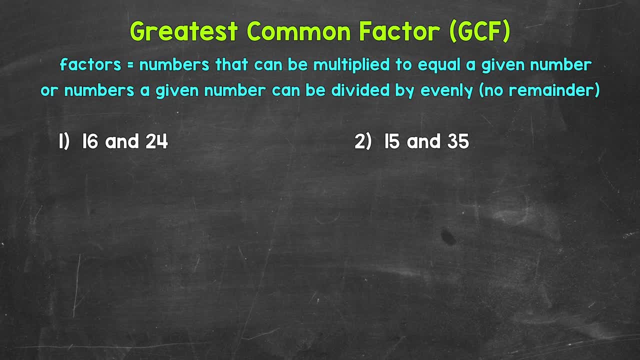 where we have 16 and 24.. We first need to list the factors of each number. Let's start with the factors of 16.. Now I would suggest always starting with the factors of one and the number itself, because we know, one times that number will equal that number itself. 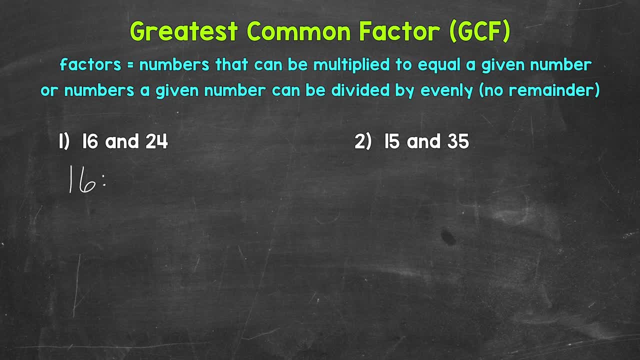 We can think of factors in terms of pairs: One times 16 equals 16.. Or we can think of it in terms of division. We can divide 16 by those factors, evenly, However you want to think about it. So I'm going to write 1 and 16 with a gap in between for the other factors. That way, 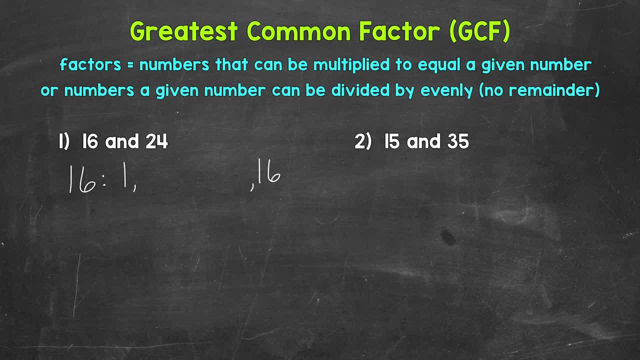 we can write the factors in order. Now we need to list the other factors as well. So let's think about what else goes into 16.. So to speak, think about multiplication facts, division facts, and we can work our way up from one. So there are different strategies and 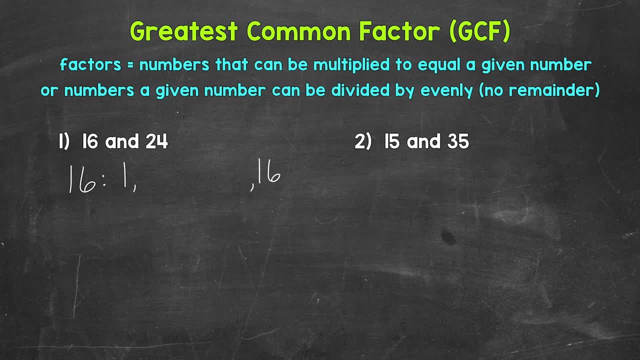 ways to work through this. The next factors of 16 are 2 and 8.. 2 times 8 equals 16.. So 2 and 8 are the other 16.. So let's think about what else goes into 16.. So let's think about what else goes into 16.. So 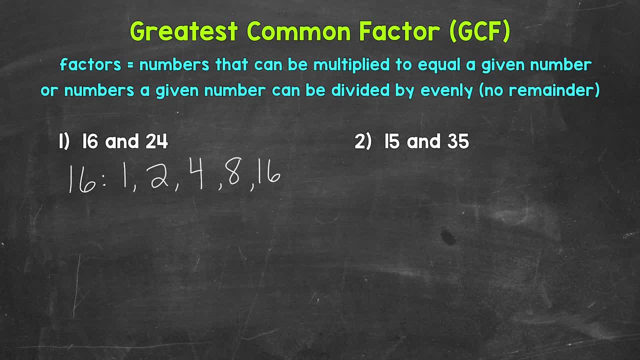 16.. And then our last factor of 16 is 4.. 4 times 4 equals 16.. So 4 is a factor of 16.. Although 4 times 4 equals 16, we only need to write 4 once in our factors list, And that's it. 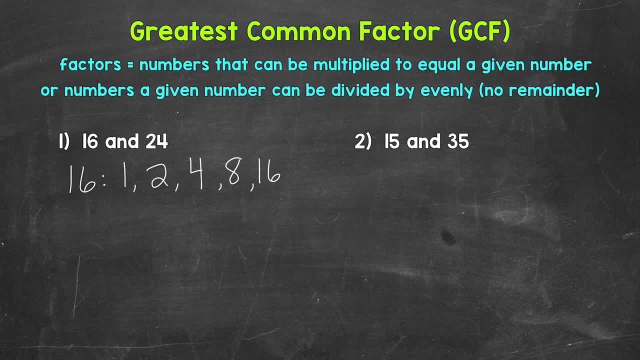 for the factors of 16.. You can always think about other possible factors if you're unsure, if you're done, For example, 3, 5, 6, and so on, But we have them all. The factors of 16 are 1,, 2,, 4,, 8, and 16.. 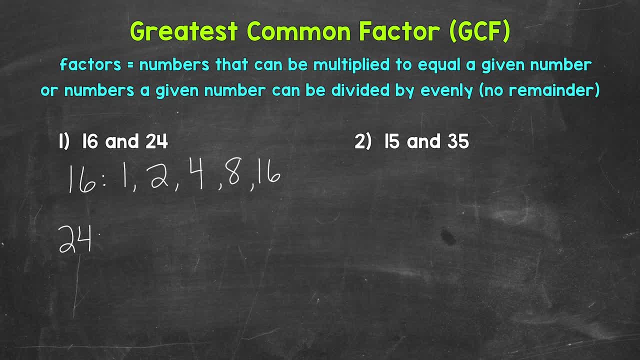 Let's move on to the factors of 24.. We will start with 1 and 24.. Next we have 2 and 12.. 2 times 12. Equals 24.. So 2 and 12 are factors of 24.. Then we have 3 and 8.. 3 times 8 equals 24.. So 3 and 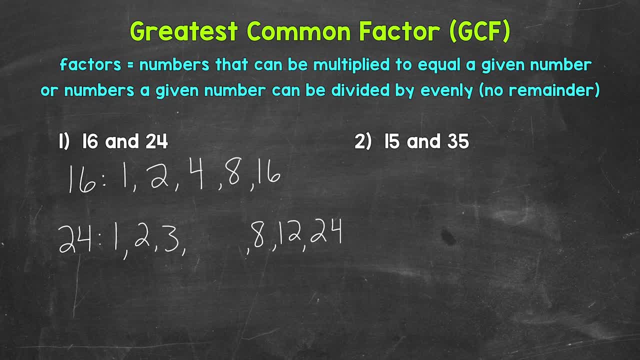 8 are factors of 24.. And then, lastly, we have 4 and 6. 4 times 6 equals 24.. So 4 and 6 are factors of 24.. And that's it for the factors of 24.. 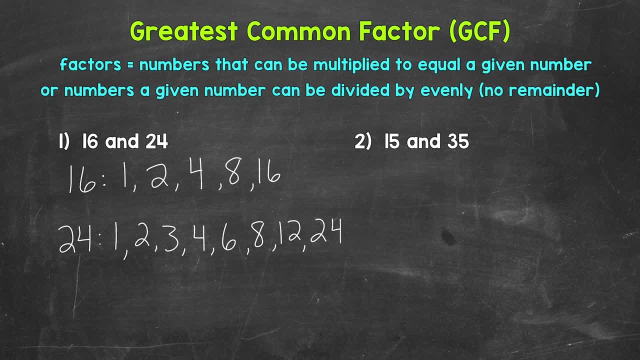 1,, 2,, 3,, 4,, 6,, 8,, 12, and 24.. Now that we have the factors listed for our numbers, we need to look for common factors and specifically the greatest common factor. So let's look for factors. 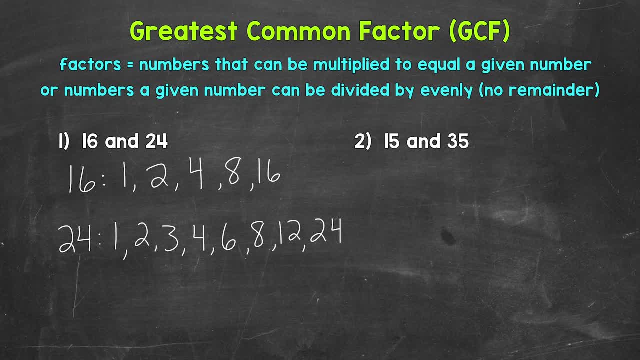 that these numbers share, that they have in common. So 1 is a common factor, 2 is a common factor, 4 is a common factor And then 8 is a common factor. So the greatest common factor is 8,. 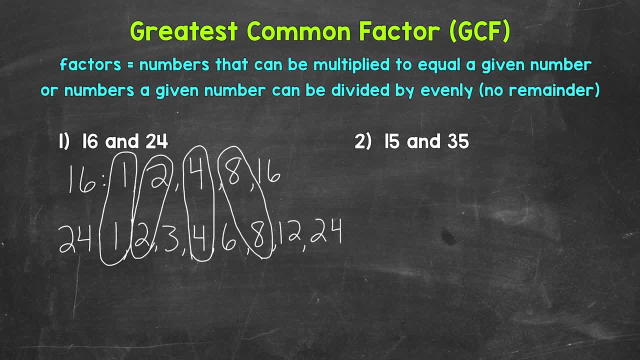 the greatest factor in value that they share, the greatest factor in value that they have in common. So the GCF, the greatest common factor is 8.. The greatest common factor of 16 and 24 is 8.. Let's move on to number 2.. 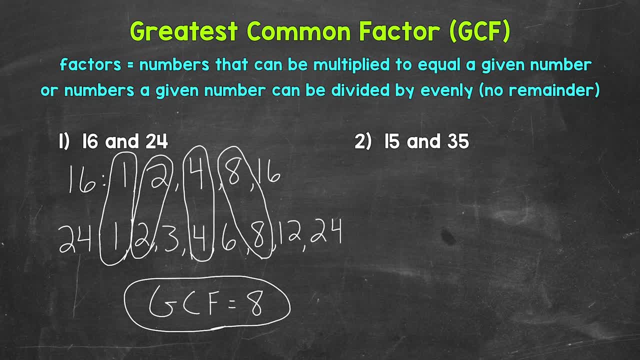 Where we have 15 and 35. Let's start with the factors of 15.. We have 1 and 15.. Next we have 3 and 5.. 3 times 5 equals 15.. So 3 and 5 are factors of 15.. And that's it for the factors of 15.. 1,. 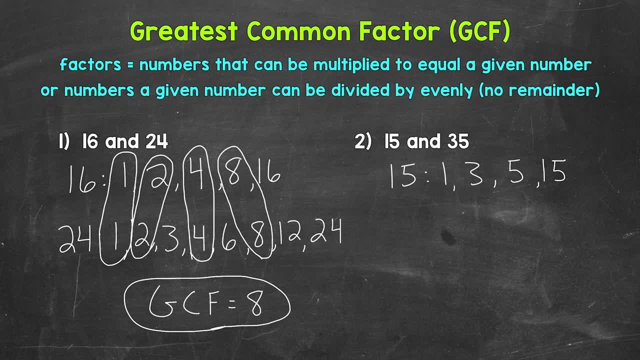 3, 5, and 15. Factors of 35. So we have 1 and 35. And then 5 and 7.. 5 times 7 equals 35. So 5 and 7 are factors of 35. And that's it for the factors of 35.. 1,, 5, 7, and 35. 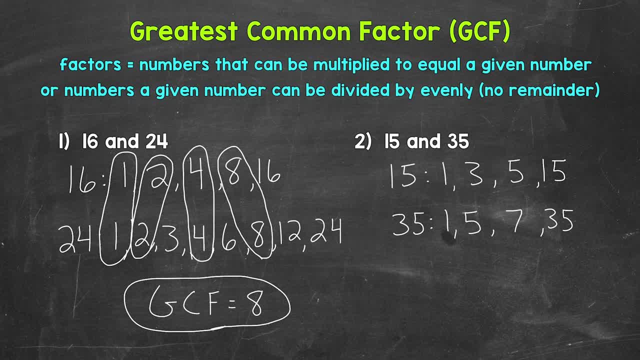 Now that we have our factors list for our numbers, we need to look for common factors and specifically the greatest common factor. So 1 is a common factor And then 5 is a common factor. That means 5 is the greatest common factor, So the GCF the greatest common factor. 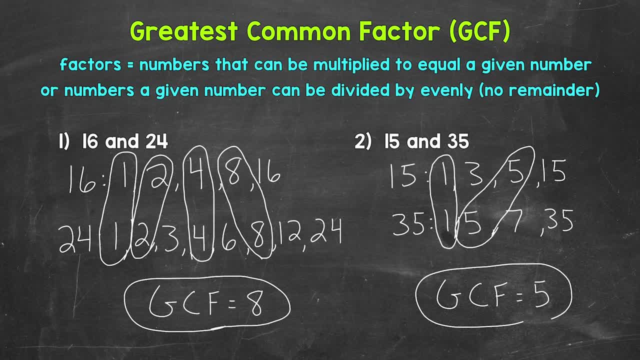 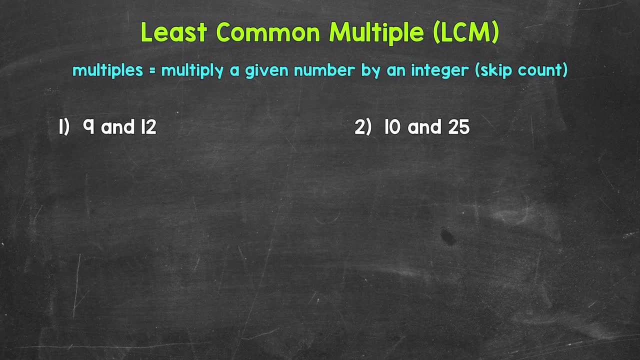 is 5.. The greatest common factor of 15 and 35 is 5.. So there's how we find the greatest common factor. Let's move on to least common factor. Here are our examples for least common multiple. Now, as far as the least common multiple between: 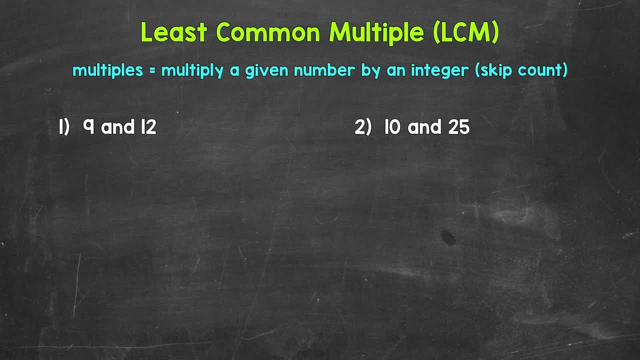 numbers. this is going to be the smallest multiple in value that both numbers share. Now, a multiple is the result of multiplying a given number by an integer. When we think of multiples of a number, we need to think about the numbers we get when multiplying. 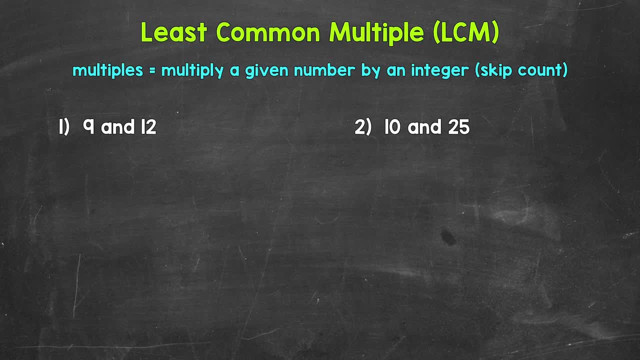 that given number by integers. A simpler way to think about multiples is to think about skip counting. So all of the numbers, something is going to hit when you count up by that number. Those are all going to be multiples. This will make a lot more sense as we go through our examples. 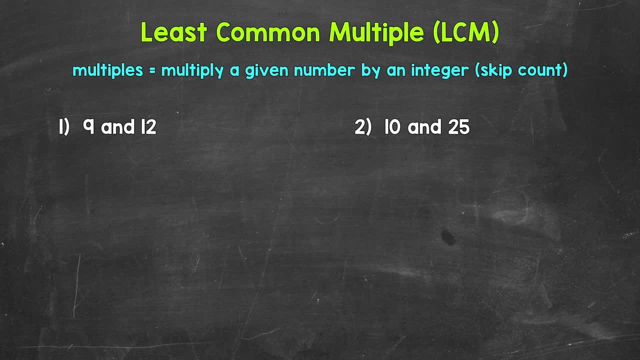 Let's jump into our examples, starting with number 1, where we have 9 and 12.. We're going to start by listing some multiples of both 9 and 12.. Then we will look for common multiples and specifically the least common multiple, also referred to as the LCM. Let's start with some multiples of 9,. 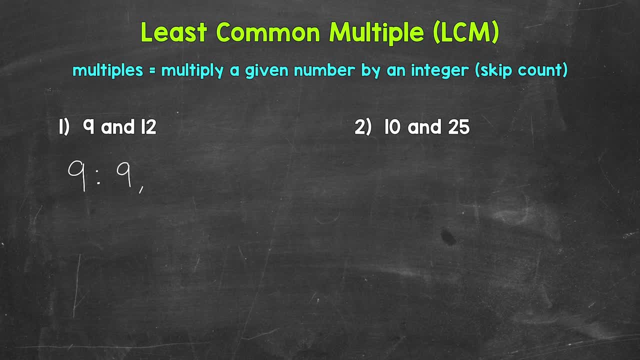 which are 9 times 1, which is 9.. 9 times 2 is 18.. 9 times 3 is 27.. 9 times 4 is 36.. And 9 times 5, is 45. So you can see that we just skip counted by 9 to list those multiples: 9,, 18,, 27,, 36,, 45,. 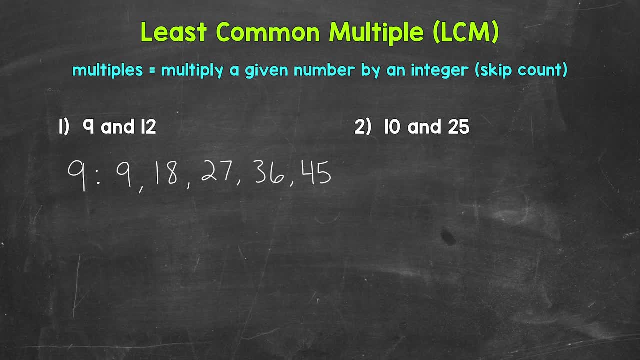 so on and so forth. Now I stopped at 45 because multiples go on forever, They are endless, They are infinite. My suggestion is to list 4 or 5 multiples when looking for the least common multiple. So list 4 or 5 multiples when looking for the least common multiple. So list 4 or 5. 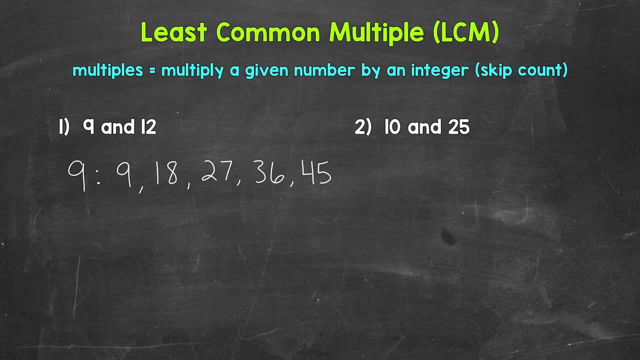 multiples for each number. Look for any in common, And if you don't have any in common, you can always extend the multiples lists. Now let's list the first 5: multiples of 12.. 12 times 1 is 12.. 12 times 2 is 24.. 12 times 3 is 36.. 12 times 4 is 48. And 12 times 5. 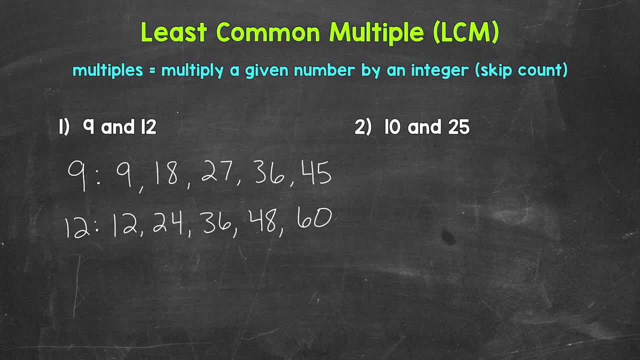 is 60. So again, you can see that we skip counted there. We skip counted by 12.. So 12,, 24,, 36,, 48,, 60, so on and so forth. Now that we have some multiples listed for both 9 and 12, we need to. 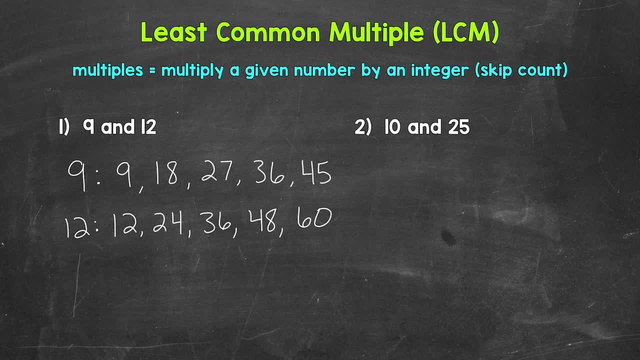 look for any common multiples, So any multiples that they share, And then, specifically, we need to look for the least common multiple. Well, 36 is a common multiple And it's going to be the least common multiple, So the smallest multiple in value that they share. So let's. 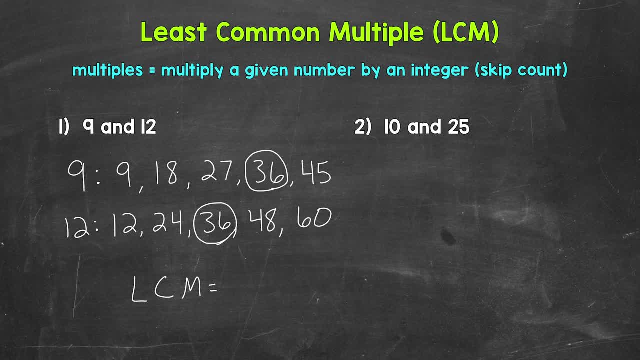 write that the LCM, which stands for least common multiple, is 36.. So the least common multiple of 9 and 12 is 36.. Now, one thing I do want to point out is that the least common multiple of 9 and 12 is 36.. 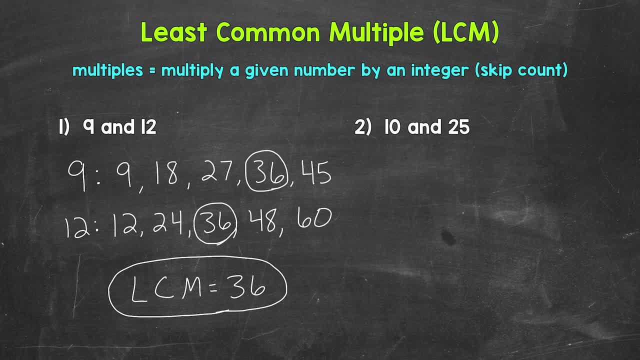 One thing I do want to mention about common multiples is that they are infinite. Although we only have one common multiple in our lists, as is 36, we can always extend multiples lists, So we can always keep going to find more common multiples. Remember, multiples are endless. 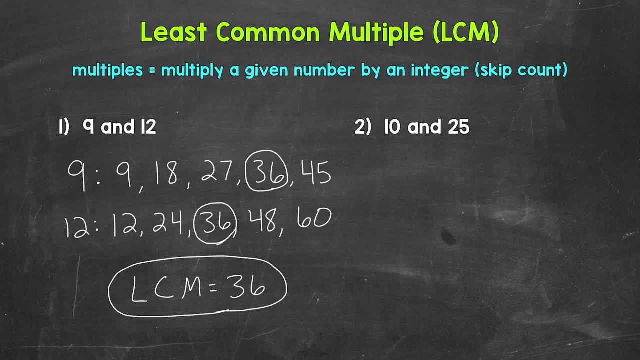 So that means common multiples are endless. So that's just something to think about. when it comes to multiples, Let's move on to number two, where we have 10 and 25.. Let's start with some multiples of 10.. So 10 times 1 is 10.. 10 times 2 is 20.. 10 times 3 is 30.. 10 times 4 is 40. And then 10 times 5. 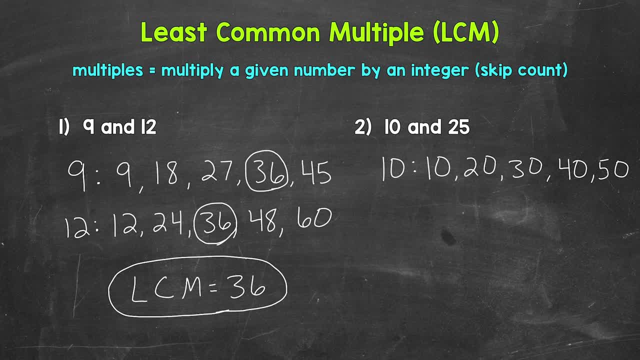 is 50.. So 10, 20,, 30,, 40,, 50, so on and so forth. Now let's list the first multiple: 5 multiples of 25.. So 25 times 1 is 25.. 25 times 2 is 50.. 25 times 3 is 75.. 25 times 4 is 100. 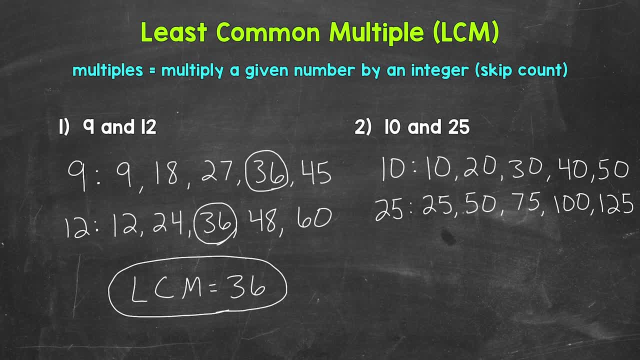 And then 25 times 5 is 125.. Now that we have some multiples listed, we can look for common multiples and specifically the least common multiple. Well, 50 is a common multiple And it happens to be the least common multiple, So the LCM is 50.. The least common multiple of 10. 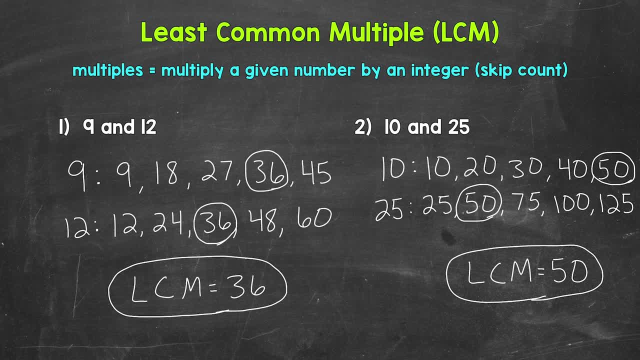 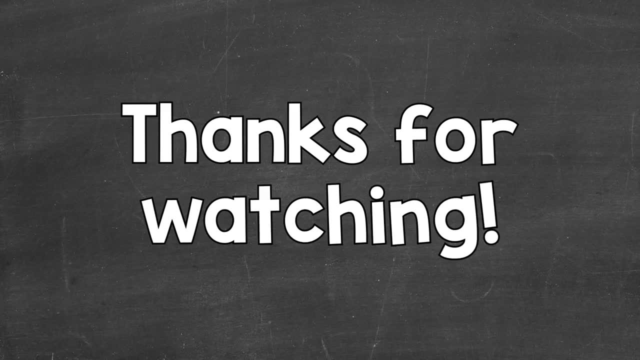 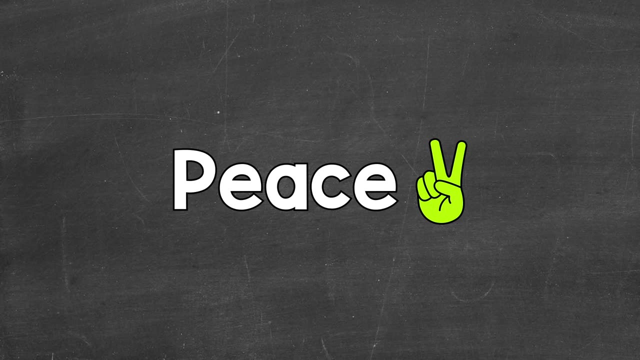 and 25 is 50.. So there you have it. There's how to find the GCF and LCM. I hope that helped. Thanks so much for watching. Until next time, peace.